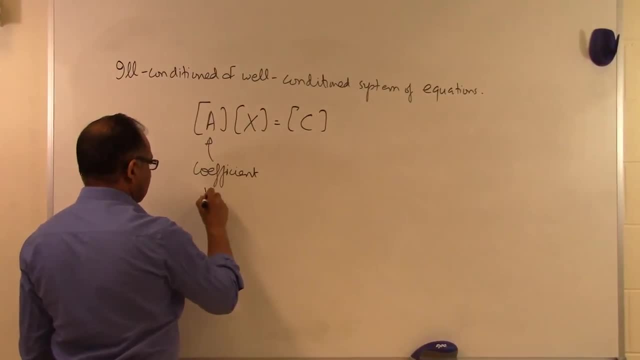 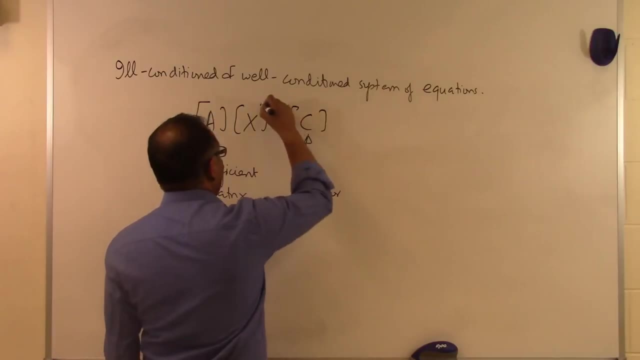 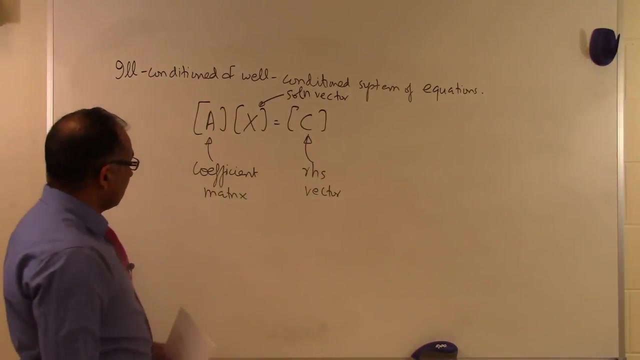 matrix, and c is the right hand side vector and, of course, x is our solution vector, or what we call as the unknown vector. So whenever we start setting up simultaneous linear equations, we write them in the form of a times x equal to c, where a is the coefficient matrix x. 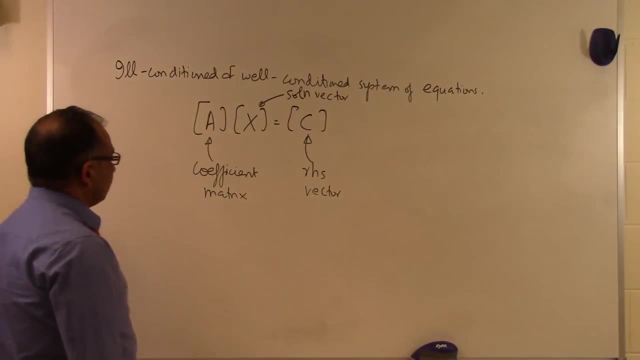 is the solution vector or the unknown vector, and c is the right hand side. What you would like to see is that, if you want to determine whether this particular system of equations is well-conditioned or ill-conditioned, is to say the following: that, hey, if I make a 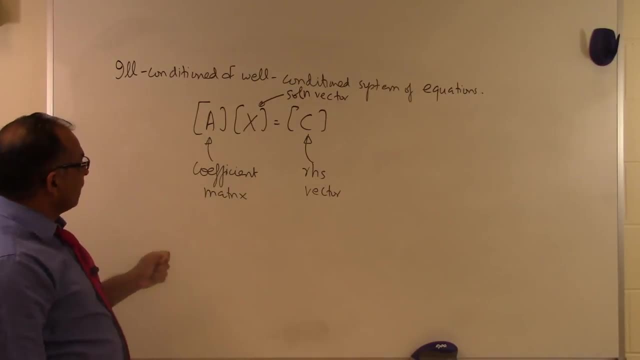 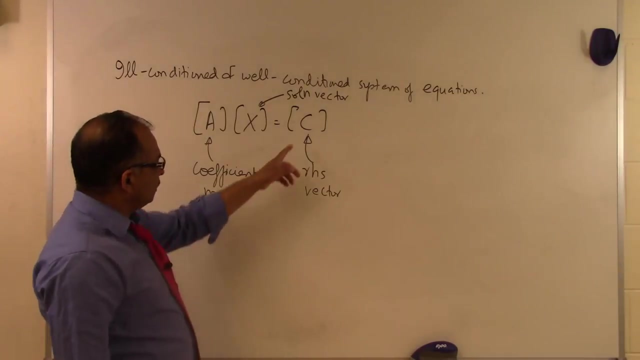 small change in the elements of the A matrix, then how much change is it making in the solution vector? or if I make a small change in my C vector, then how much change does it make in my solution vector? because you would like that, hey, if I make a small change in the coefficient, 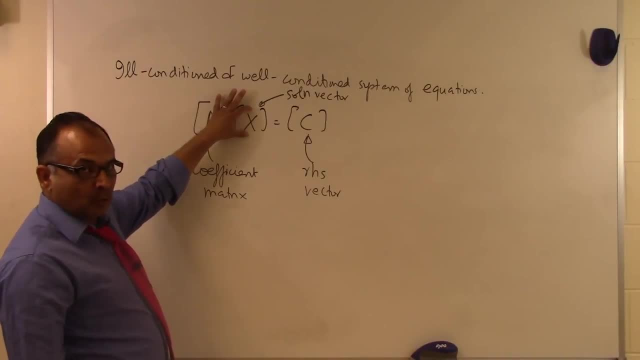 matrix, You would like the solution vector to change in a small amount. or, if you change the right hand side vector, you would like the solution vector to also change by a small amount, because we're going to, as we go through the process of setting up simultaneous linear equations, 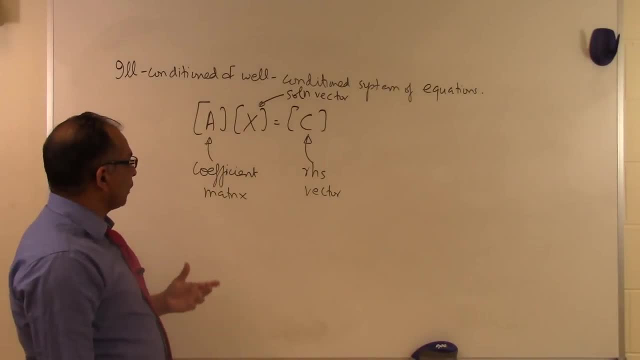 for real life problems. those might be set up through a program where we're going to have round off errors in the calculation of A matrix and the calculation of C matrix. let's suppose We don't want such round off errors or the lack of our use of precision. We want 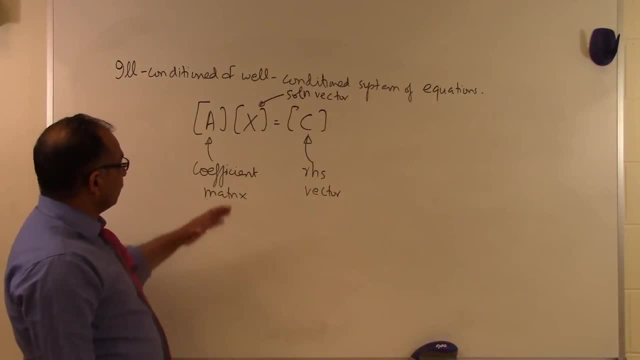 to use only single precision rather than double precision or chord precision to effect adversely what the solution vector is. and if it does, we want to have a mechanism of knowing whether it is doing so. So let's look at some examples right here to see that, whether you can see. 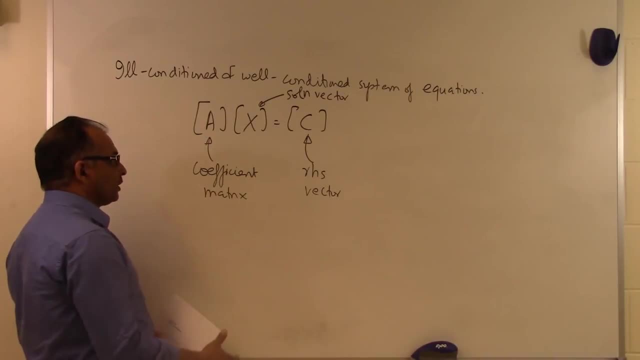 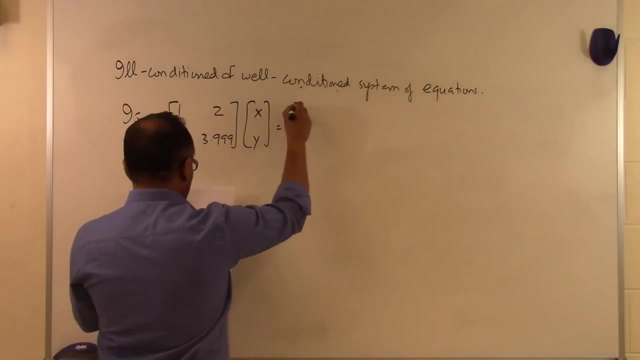 that from a simple example whether a system of equations is well-conditioned or ill-conditioned. Let's suppose somebody says: is this particular system of equations- one, two, two, three, four, seven point, nine, nine, nine, x, y is equal to four, seven point nine, nine, nine- well-conditioned? 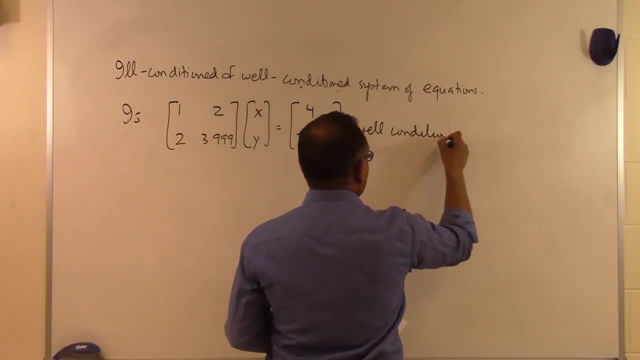 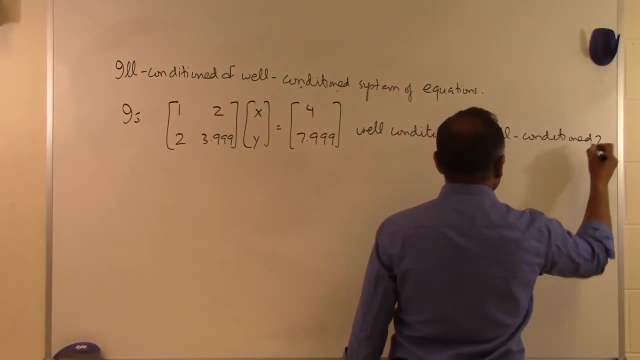 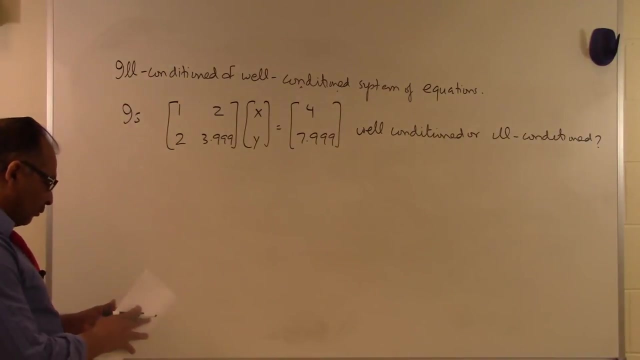 or ill-conditioned. So we want to be able to make the difference between saying that, hey, if somebody gives me a system of equations like this one, is it well-conditioned or ill-conditioned. I can see that if I wanted to solve this set of equations. 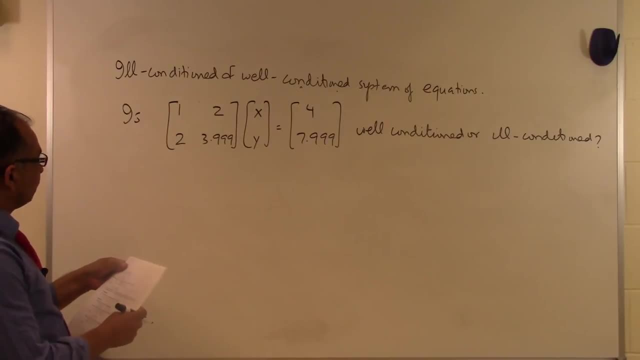 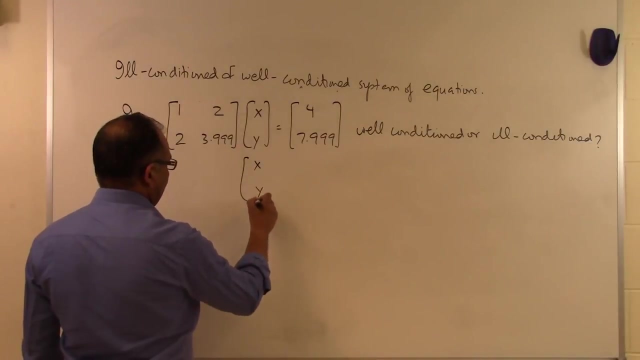 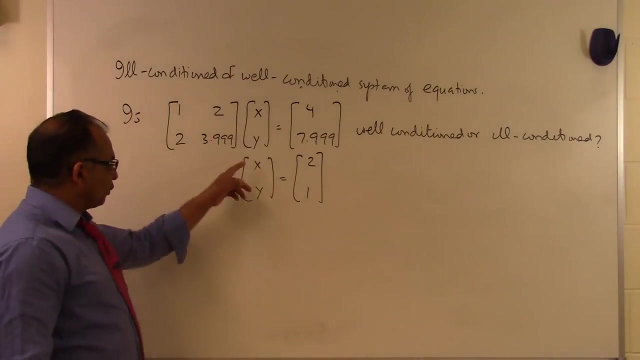 It does have a simple solution. for example, What is the solution to this one? It's two comma one, So x comma x. y is two comma one, So x. if you take x equal to two and y equal to one, In fact, if you plug x equal to two and y equal to one in here, you will get four. 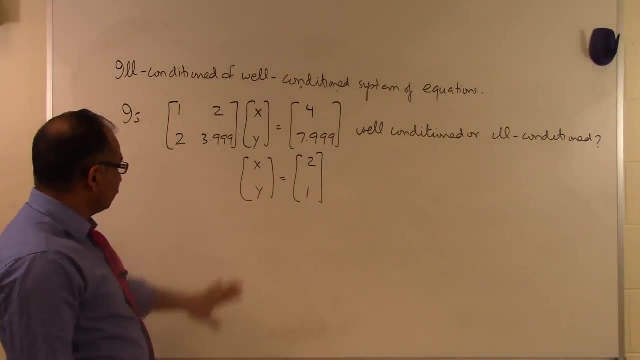 and seven point nine, nine, nine. So that's itself the solution for that and we want to see that, whether if a small change in the coefficient matrix is it going to result in a very difficult situation, A different value of x and y I'm going to get, or if I make a small change in my right. 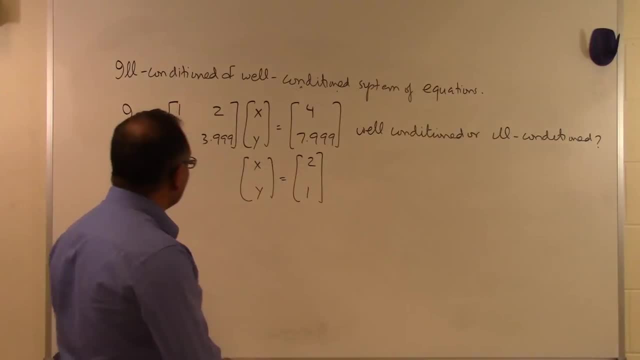 hand side vector, is it going to make a big difference in my x and y? And what I'm doing now here is, let's suppose I make a small change in my coefficient matrix. So what I'm doing is as follows: I'm taking one point, zero, zero one, So I'm making a small change in the coefficient. 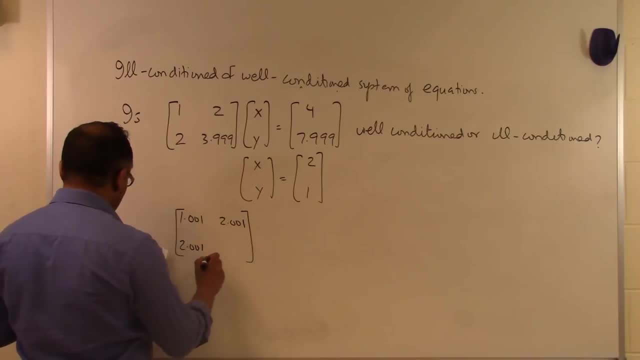 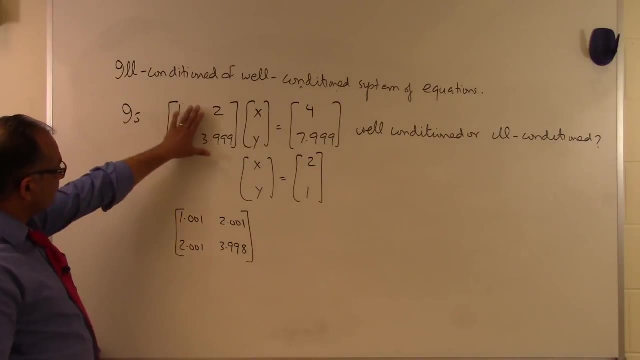 matrix, changing it by the thousandths. So I get three point nine, nine, eight. So what I'm doing is that I'm making a change of about a magnitude of point zero, zero one for all of these elements which are right here in the coefficient matrix, And I will not 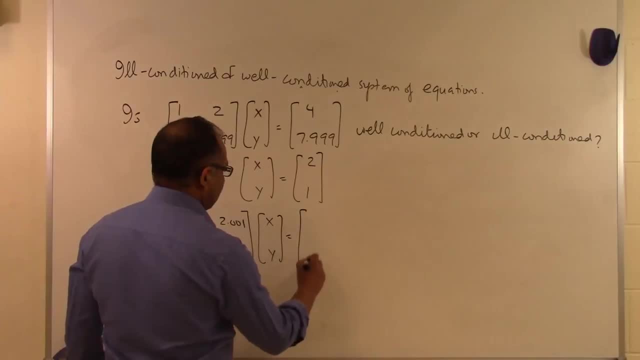 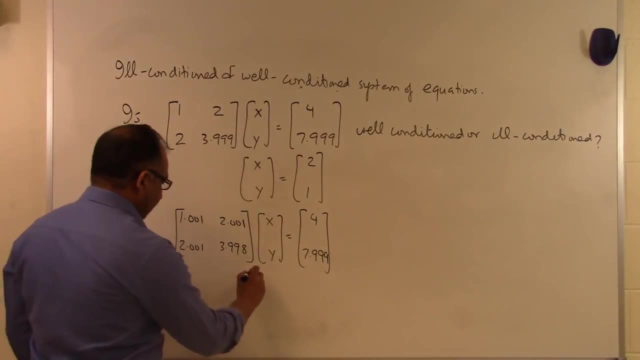 change the right hand side, And I want to see that. hey, does it make a big difference in my solution? And what I find out is that, hey, if I solve these two unknowns by hand or by using MATLAB or any kind of calculator, The answer which I get is as follows: Three: 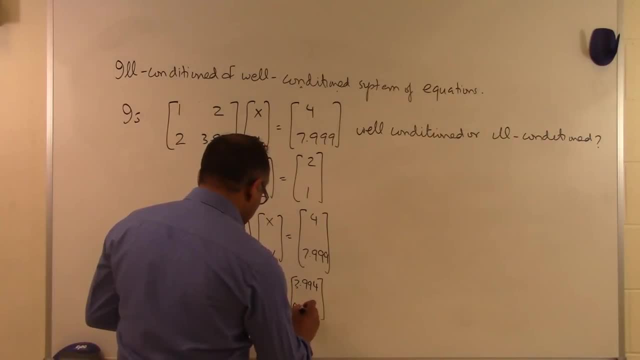 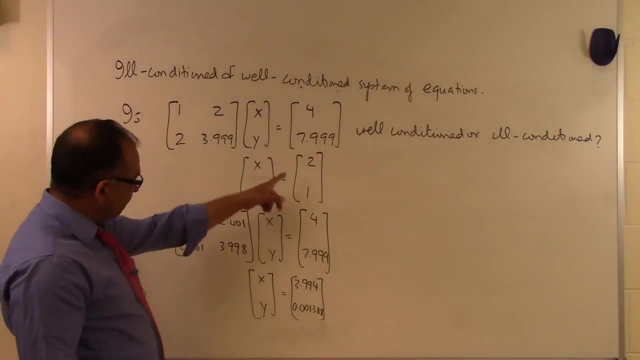 point nine, nine, four. zero point, zero, zero one. three point nine, nine, four. So that's three, eight, eight. And you can see that just by watching it or just by looking at it, you can see that this value of two has changed to almost four. This value of one has changed. 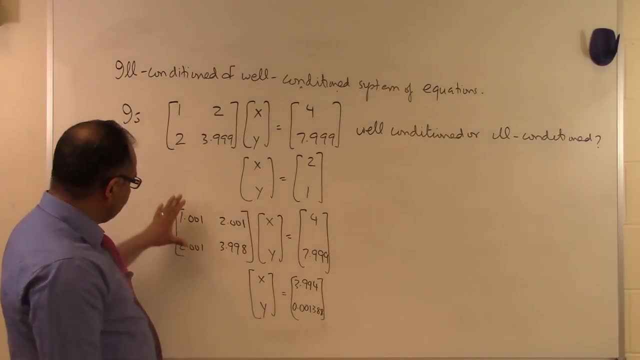 to almost a value of point zero, zero, one So very different, with very small change being made in the coefficient of the A matrix. So we can very well see that, hey, this is not a well conditioned system of equations. In order to complete the argument, let's go and: 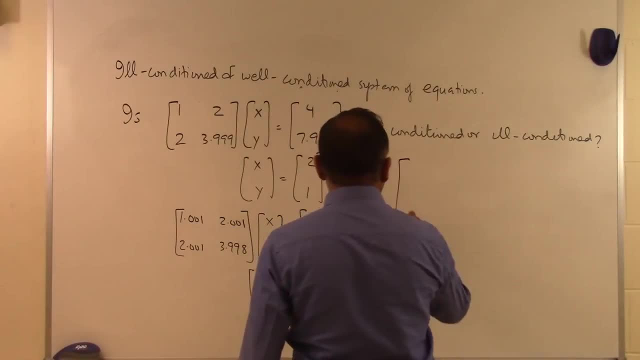 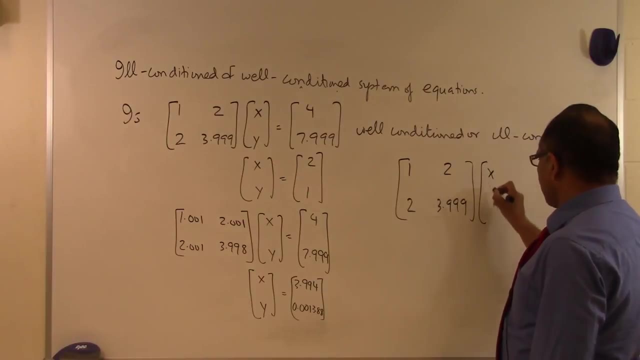 change the right hand side a little bit. So let's suppose I have one, two, three, point, nine, nine, nine here, And what I do is I keep the coefficient matrix the same, But I change the right hand side a little bit. So let me. 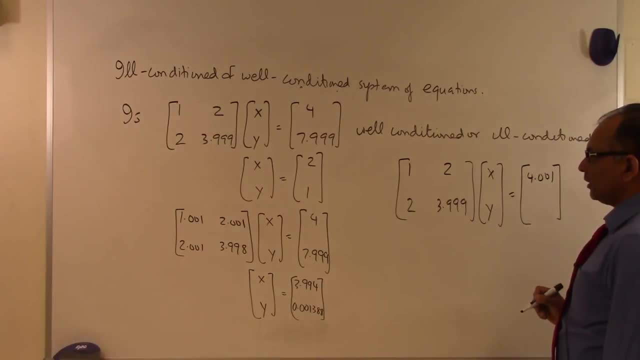 make this to be again one thousandths of difference there, And seven point nine, nine, nine, eight here. one thousandths of a difference right there. And let's go and see what I get for value of x and y. So I get x and y here And if I calculate the value I get one thousandth. 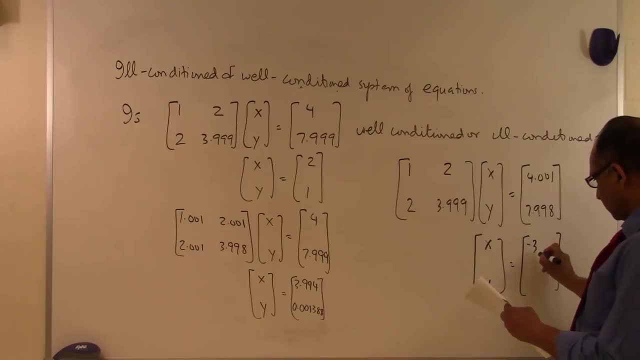 of a difference Minus three point nine, nine nine and four point zero, zero. So again, you are finding out that from the original set of equations which we had right here, where the solution was two and one, I made a very small change. I changed four to four point. 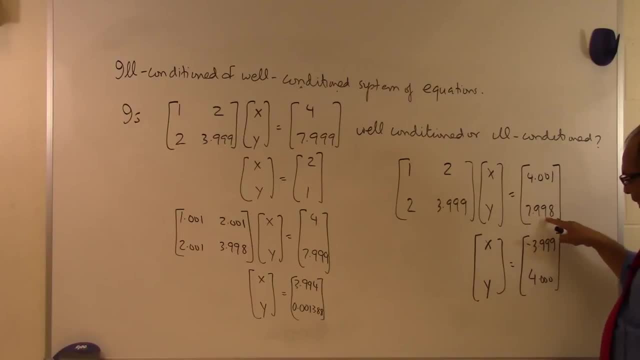 zero, zero one. I changed seven point nine, nine nine to seven point nine, nine, eight. Just a small change, A small relative change in the coefficient In the right hand side. So that's what I get. So this is the value of x and y. So this is the value of x and 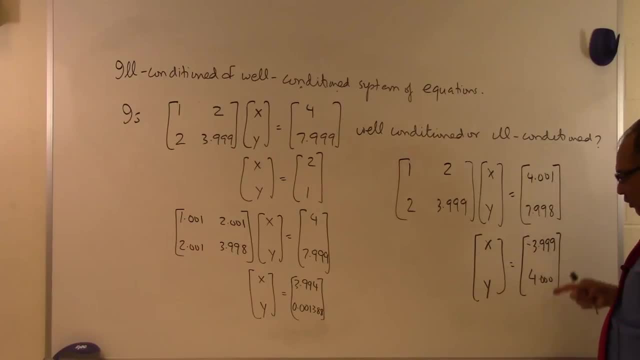 y And put it in the right hand side vector. But when I solve these two equations to unknowns by using Imprisoned Math Lab, whatever you find out that the solution which I get is different. This was two, Now it is minus three point nine. nine, nine. This was one, And now. 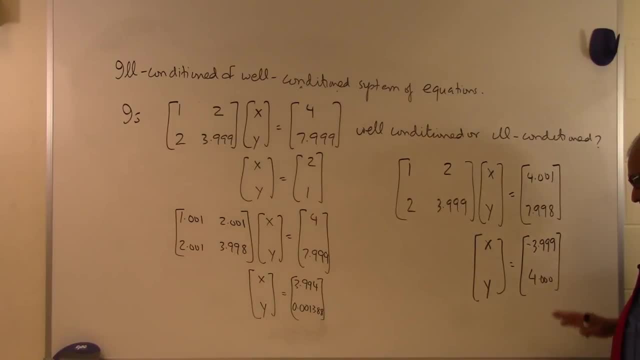 it is becoming four. So if somebody had to ask me Just by intuition: Is this a well conditioned system of equations or ill conditioned system of equations? I would term this to be ill conditioned system of equations. Now, in the later segments we will talk about how do we do this. by now, For every equation, we will make it to them here, In this example, what we have. 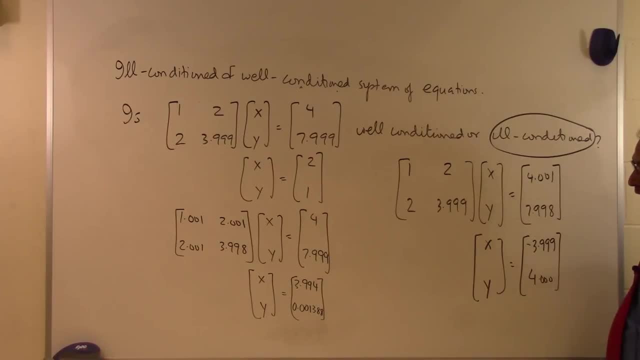 is the value of y, One thousandth of a difference. But now we are offhand. Let me get it to east of half segments we'll talk about how do we do this quantitatively without having to do this. But as an illustration to illustrate the point that hey, what does it mean that a particular 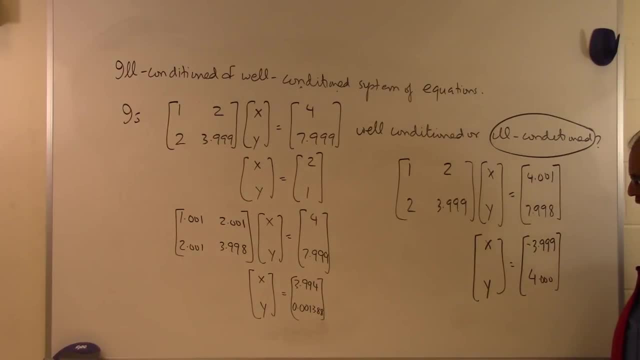 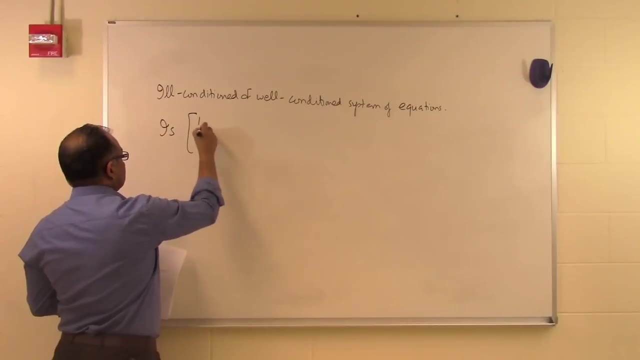 system of equations is well conditioned or ill conditioned. This is a very good example to follow. Let's see if this system of equations is 1,, 2,, 2,, 3,, x, y, well conditioned. This system of equations, is it well conditioned or ill conditioned? So we just want to illustrate. 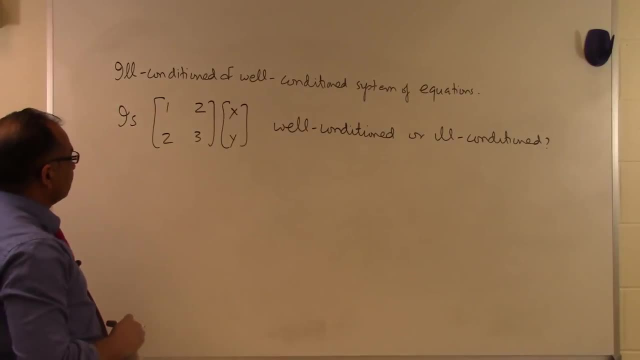 the fact whether it is well conditioned or ill conditioned. So if you look at- so I didn't put the right side here- This should be 4 and 7.. So if we have this system of equations, is it well conditioned or ill conditioned? The solution to this set of equations, if you? 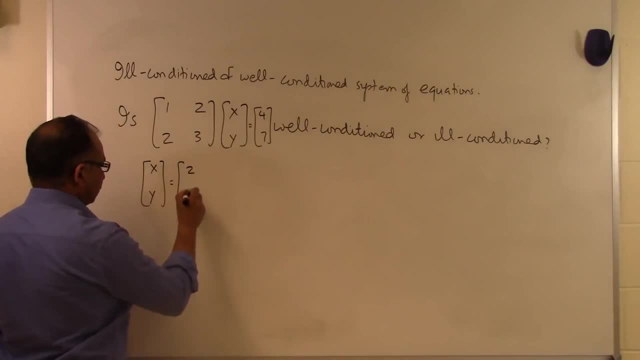 would either solve it or plug in these values of x equal to 2 and y equal to 1, you are going to get 4 and 7. or, if you solve these two equations, two unknowns, you're going to get x, y equal to 2 and 1.. In order to find out whether this particular system of equations is well conditioned, 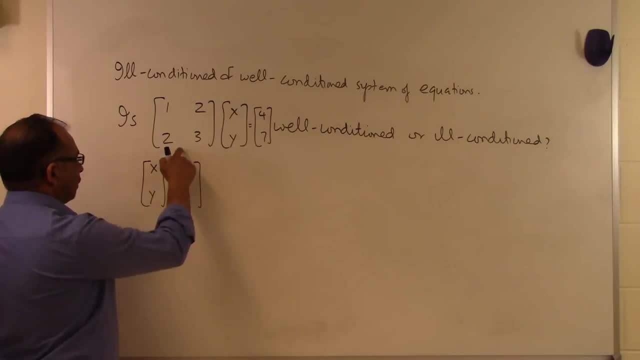 or ill conditioned. I'm going to conduct two experiments. I'm going to make a small change in my coefficient matrix. So let me make a small change in my coefficient matrix. I'm going to make 1000.. I'm going to make 2 to be 2.001.. I'm going to make this to be 2.001.. I'm going to make. 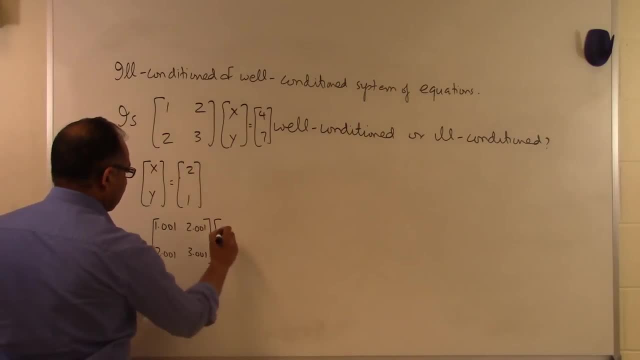 this to be 3.001.. And I'm going to say x, y is equal to 4 and 7.. So I've not made any change to the right hand side, but I've made a very small change to the coefficient matrix right here by changing the coefficients by a thousandths, And so what I get is x1 is. 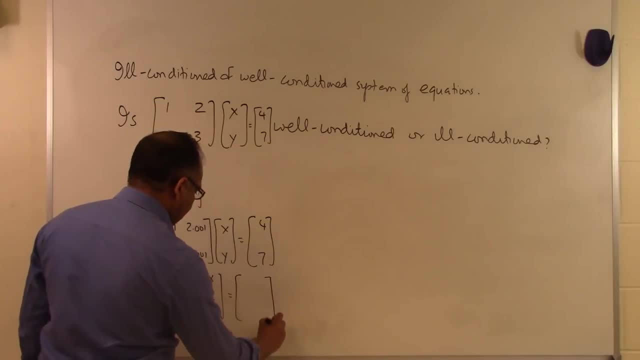 y. when I solve these two equations, two unknowns, by hand or by calculator or by MATLAB, I get 2.003 and 0.997.. And you can very well see that 2.003 is very close to. 2.0.0997 is very. 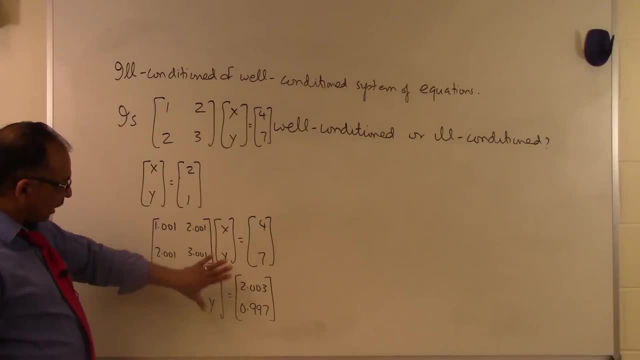 close to 1.. So a small change in the coefficient matrix did not result in a large change in my solution vector. A small change in the coefficient matrix resulted in a small change in my solution vector. Let's, for sake of completion of the experiment, let's go and